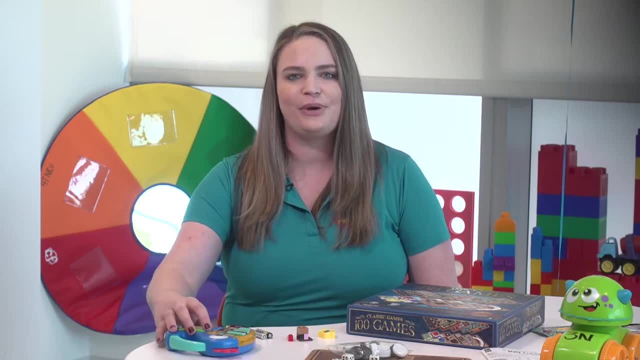 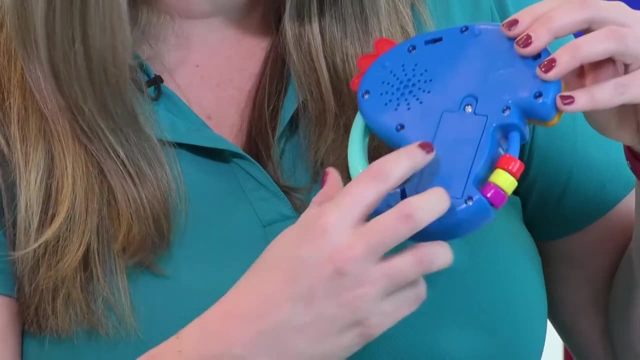 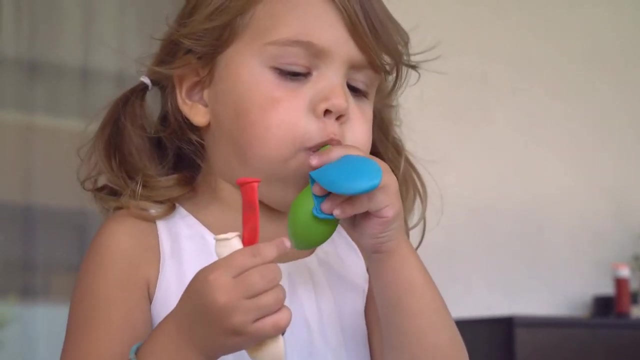 These can accidentally strangle them. Electrical toys are a potential burn hazard. Make sure the battery compartments are screwed properly closed, with the safety screws firmly in place. Don't let children under age eight blow up balloons. These are a choking hazard for young children trying to inflate a balloon, often in hail when the balloon is pressed to. 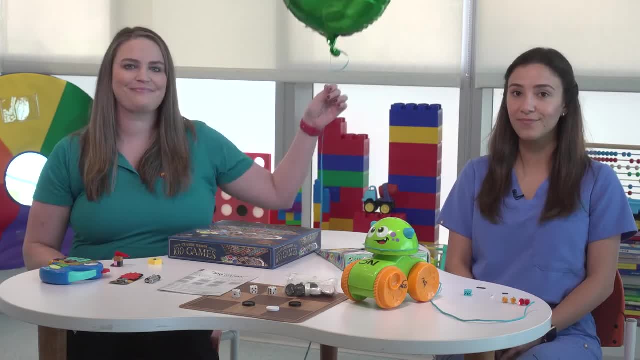 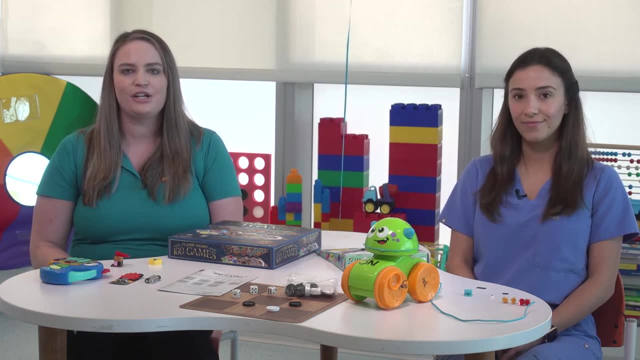 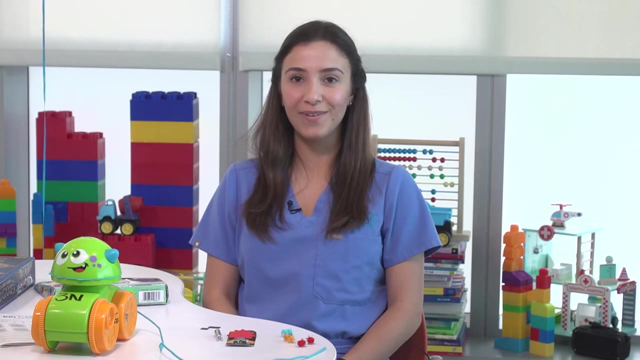 their lips. Use mylar balloons instead of latex balloons. Inspect all toys regularly for potential hazards. Check for damage that could create small pieces that are choking hazards. Additionally, in our emergency department, we often care for children with injuries caused by putting small. 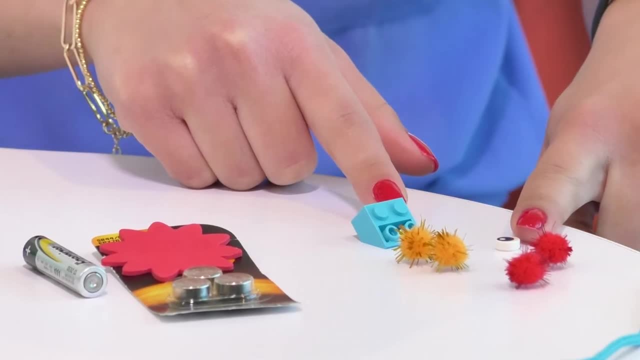 toy pieces in their nose or ears, or who have swallowed a piece of a toy. It is important to keep magnets and batteries in place. If you have a toy that is too small for your child to hold, you may want to remove the magnets and batteries out of your child's reach, as these can potentially 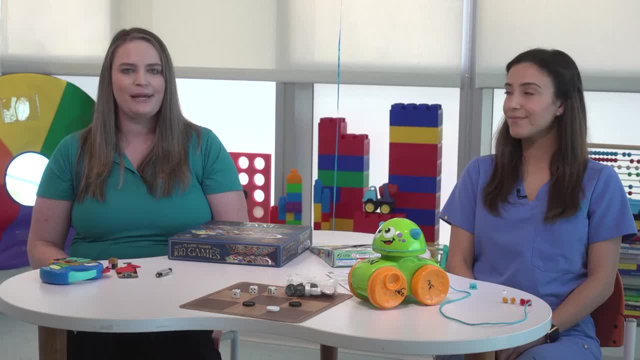 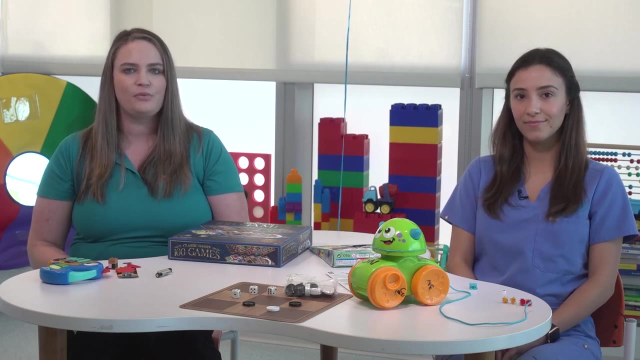 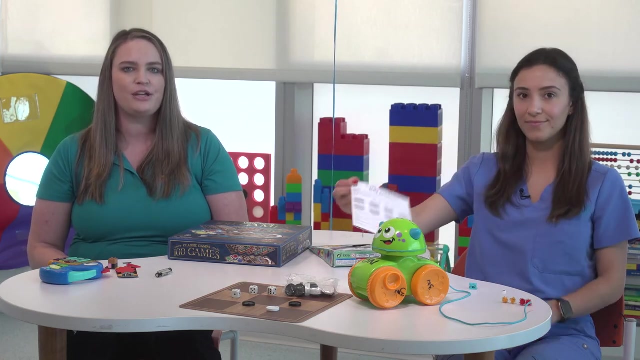 cause harm when swallowed. Make any necessary repairs immediately or discard damaged toys. Inspect all toys regularly for potential hazards. Check for damage that could create small pieces that become choking hazards. We recommend you return warranty and product registration forms for new toy purchases to manufacturers to ensure you will be notified of any recalls. 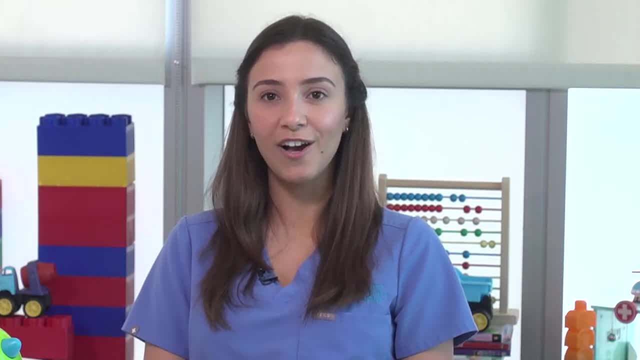 Store toys in a safe place. Put all toys away and off the floor when they are not being used. Teach your child to put toys away after playing to avoid tripping and falling over toys. Make sure that toys intended for younger children are stored separately from those for older. 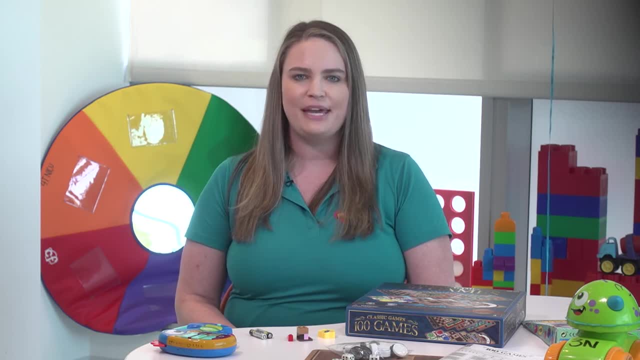 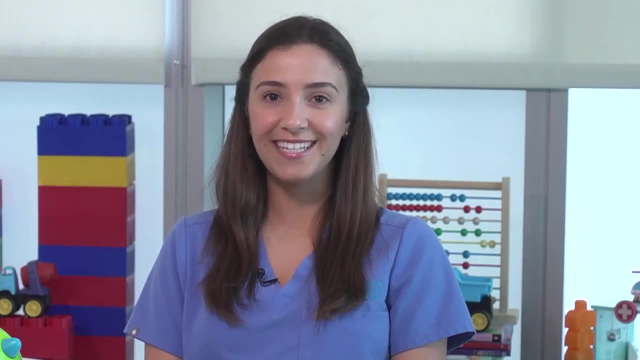 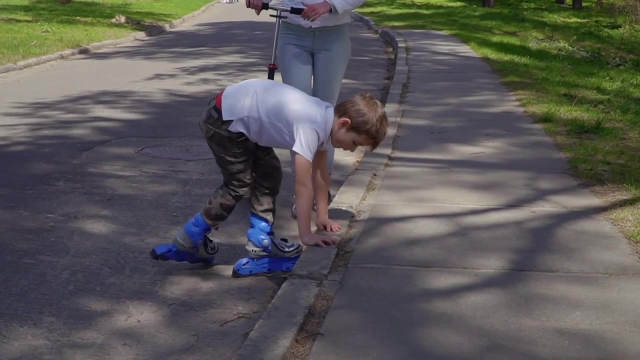 children. If storing toys in a toy chest, make sure it has safety hinges and is easy to open from the inside. Ensure that toys are used in a safe environment and with safety equipment when appropriate. For example, riding toys should not be used near stairs, traffic or swimming pools. 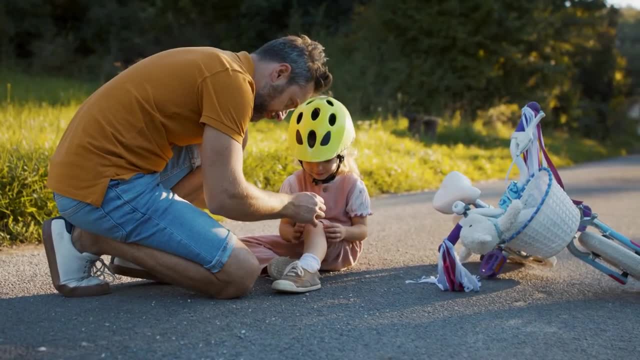 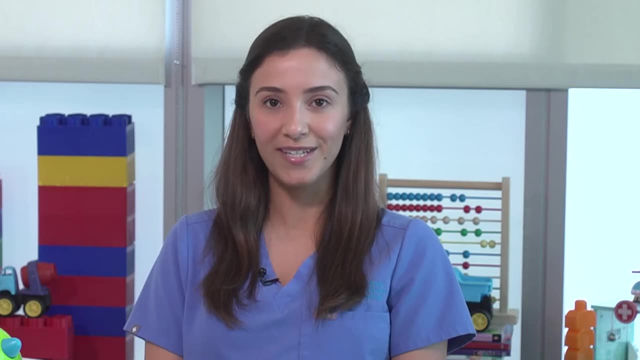 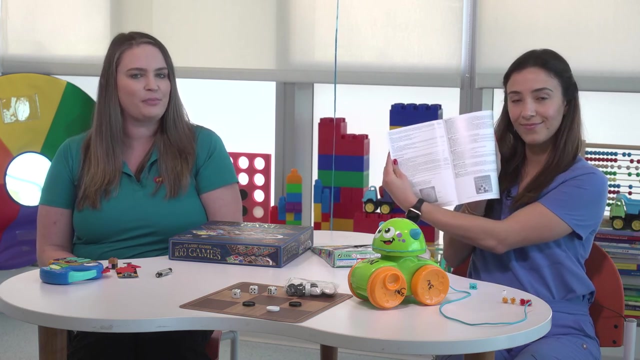 Children must wear helmets when using tricycles, bikes, scooters, etc. even if the child knows how to ride these. Many traumatic brain injuries occur due to falls involving wheeled toys. Read the toy instructions prior to your child playing with a toy to ensure it is appropriate.